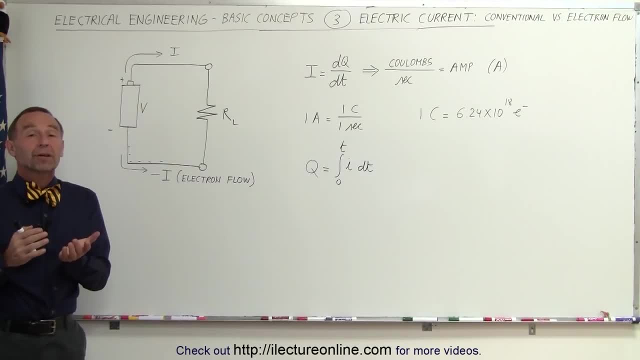 Welcome to Electro-Online. One of the most confusing aspects of Electro-Engineering versus basic science and physics, when we talk about current, is: what is the direction of the current? Well, the conventional direction of the current is that current flows from a power source and from: 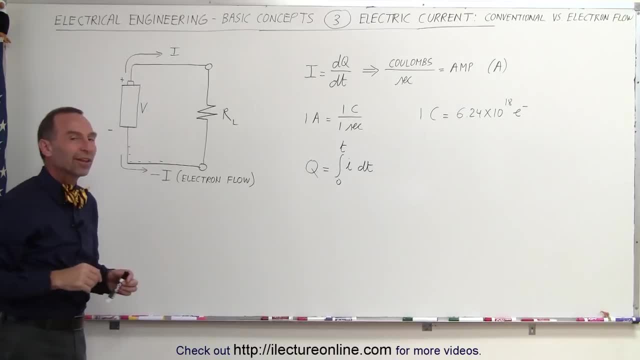 the positive end of the power source to the negative end of the power source. That's the conventional current. That's basically the current concept set up by Benjamin Franklin. He claimed that there's positive charges flowing through the circuit. However, at the time, 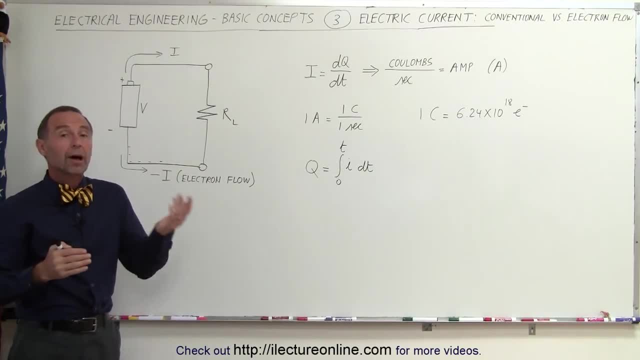 we didn't understand what the positive and negative charges were. We knew there were positive charges. We knew there were negative charges. We didn't know which ones were flowing through the circuit. The assumption was made let's just call it the positive charges. 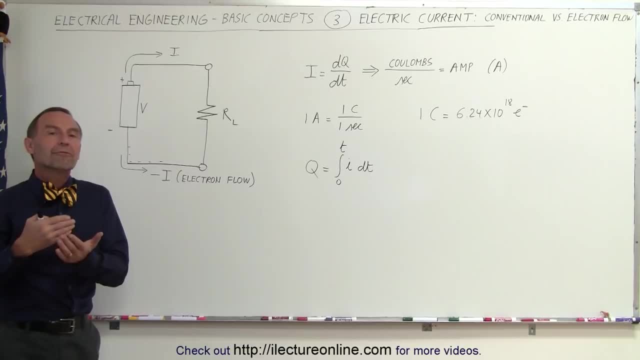 moving through the circuit. We call that the IEEE convention. It is the conventional direction of the current from positive to negative. However, we all now realize that it's the negative charges that are actually doing the moving. It's the negative electrons in the atoms of material that are moving through the circuit. in essence, the current, the 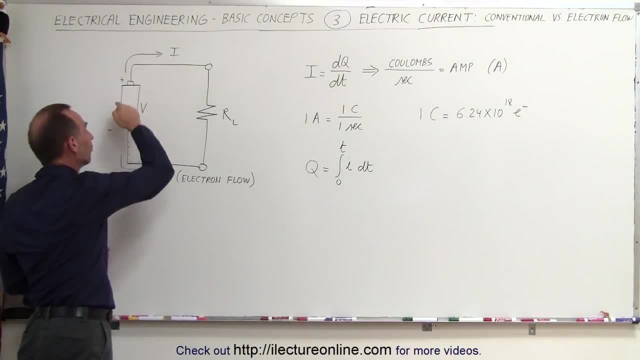 real current, the real charges are moving in the opposite direction, from the negative end of the battery to the positive end of the battery through the load resistor. what we're going to do from now on is we're going to assume that the positive current, the conventional current, is flowing. 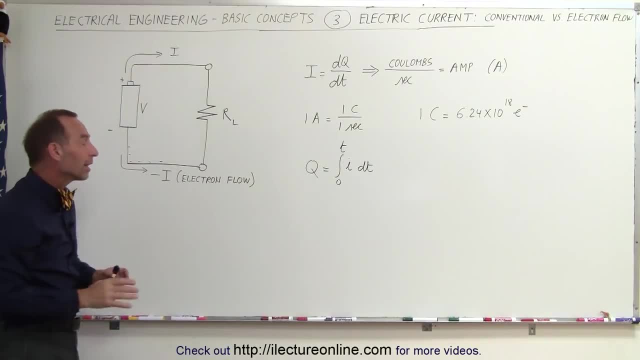 indeed from the positive to negative side, while we understand that the electrons are flowing in the opposite direction and the electrons then form the negative current. so that way we're always safe. we can say: the conventional current runs from, or flows from positive to negative and the electron 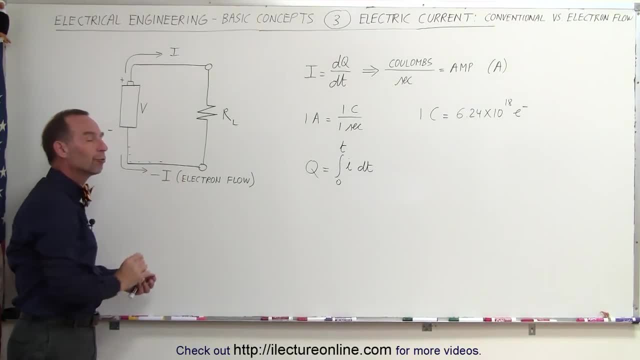 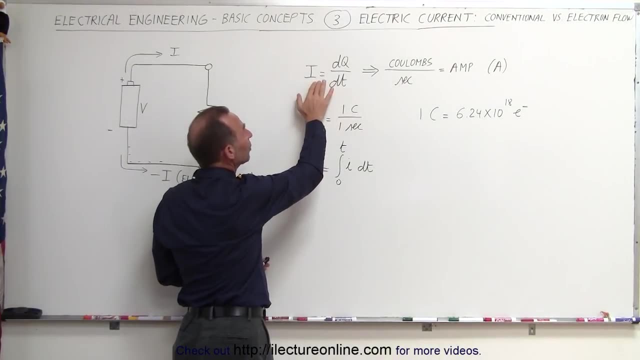 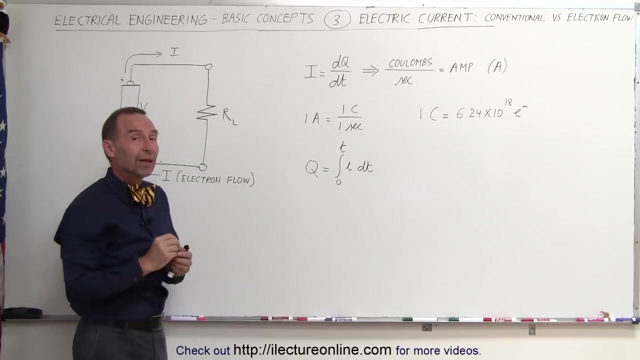 current flows from negative to positive and we call that therefore the negative current. the definition of the current is defined here by this differential equation that i is equal to the change in the charge per unit time. we really don't mean the change. we mean the amount of charge is slowing past, past a particular point. 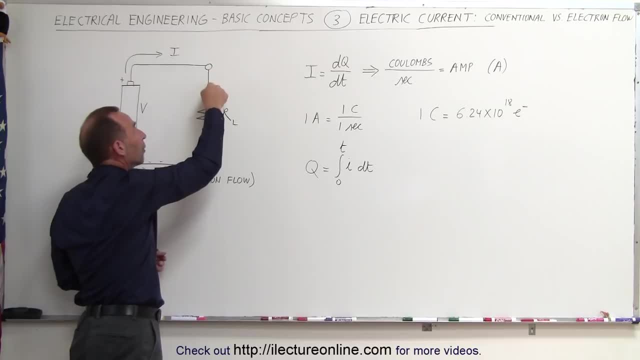 so if we take any point on the circuit and we watch current going by that point, we can say that the current flow is equal to the amount of charge that passes that point per unit time. the charge is usually indicated in terms of coulombs and the time in seconds. so coulombs per second then gives